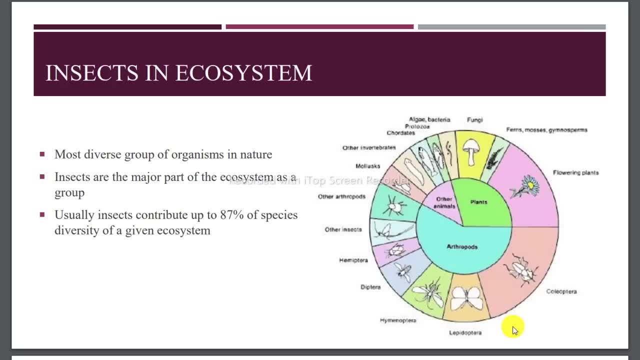 These are the types of the insects. These are the types of the insects. These are other animals, These are plants, These are arthropods. These are explained about them. These are told about them. These are told about the names of insects. You can study them. 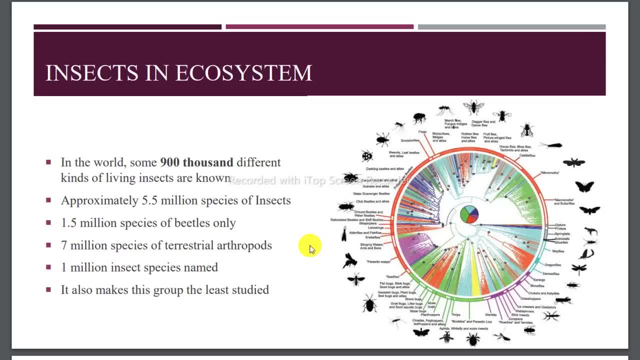 So next comes our insects in ecosystem. These are all insects. Our insects have been shown here. These are flies, ants and all kinds of insects like butterfly, etc. These are all the insects which are found in our ecosystem. It is not explained about them, but they are mostly found in agriculture lands of Pakistan. 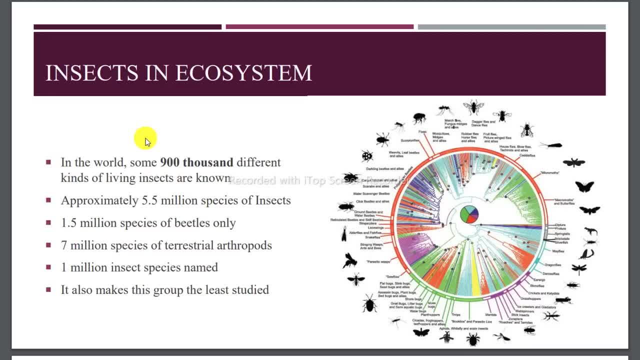 So we can study about them and find out their key points. In the world, some 900,000 different kinds of living insects are known. The world has more than 900,000 different kinds of living insects, So what are the key points in this world? 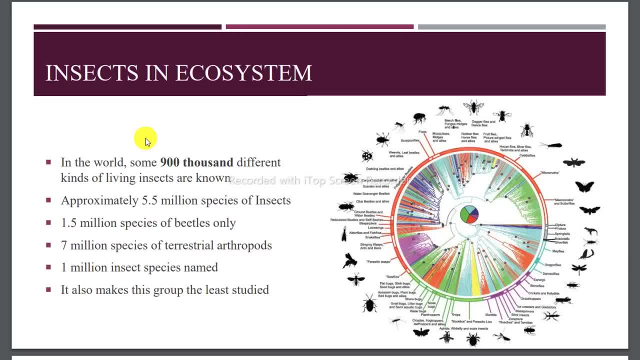 So what are the key points in this world? So what are the key points in this world? There are more than 9000 species of insects, Approximately 5.5 million species of insects, Approximately 5.5 million species of insects, 1.5 million species of beetles only. 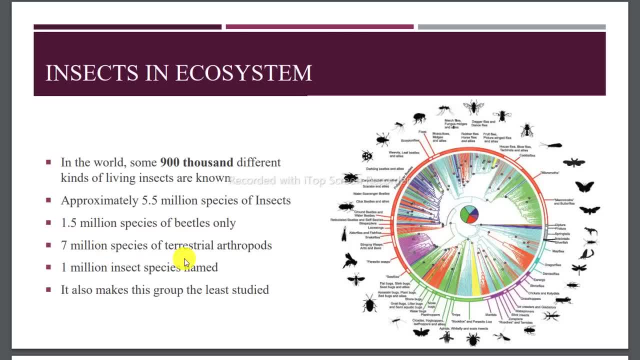 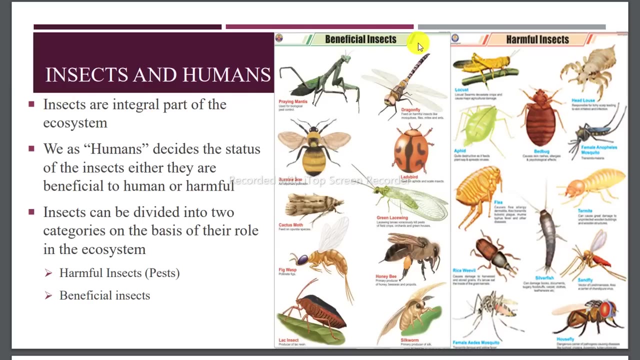 7 million species of terrestrial arthropods, 1 million species of insects. It also makes this group the least study Insects and humans. Beneficial insects and harmful insects- In our language we say Boond, Locust. All these names show Which are harmful and which are beneficial. 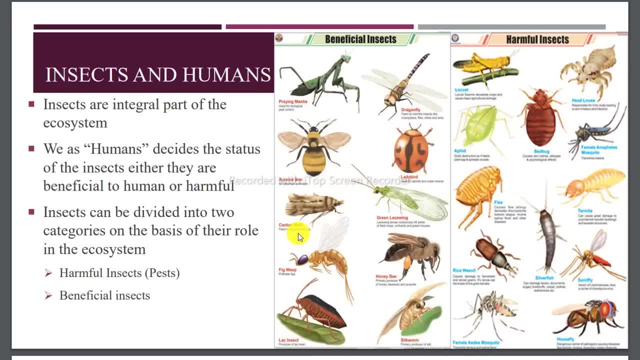 Ladybug, Bumblebee, Cactus, moth, Fly-breast, Honey bee, Many other insects, Praying Mantis, Dragonfly- All these are beneficial insects. Let's start from the first point: Insects are an integral part of the ecosystem. Insects are a very important part of the ecosystem. 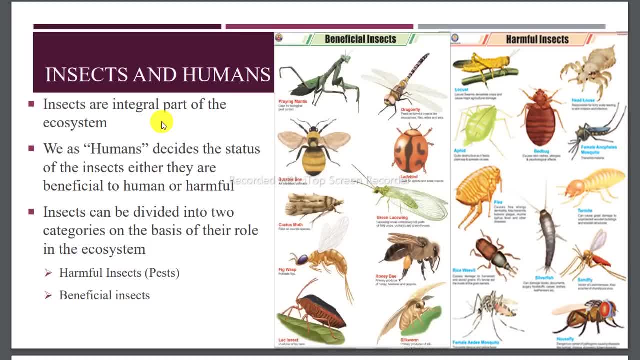 Human decides the status of the insects. Either they are beneficial to humans or harmful. We humans have decided which insects are beneficial to humans Which are harmful. Third, Insects can be divided into two categories. Insects are divided into two categories On the basis of their role in the ecosystem. 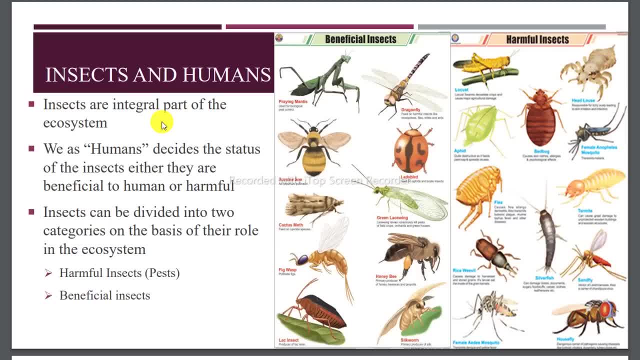 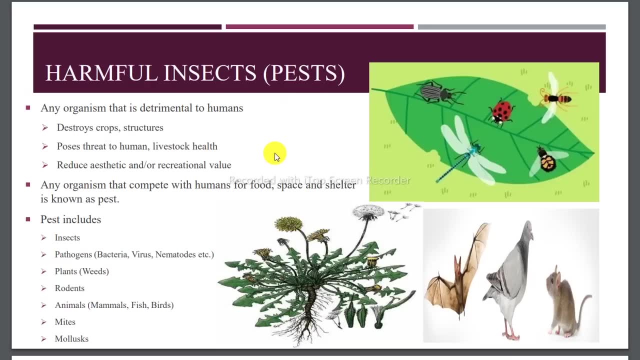 According to their role in the ecosystem Which they are performing in the ecosystem. First is the harmful insects. Second is the beneficial insects. We have read this further. Which are the beneficial insects? Which are the harmful insects? Let's talk about them. Harmful insects, Which are also called pests. 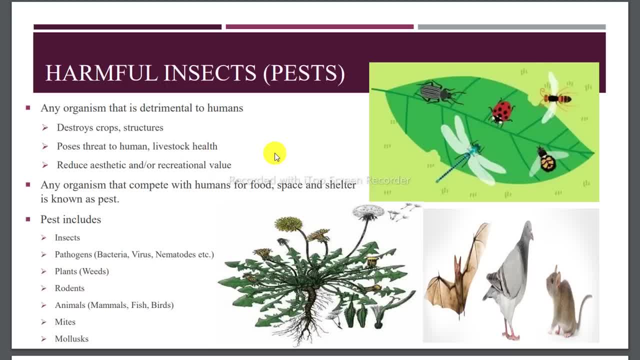 Any organism that is detrimental to humans, Destroys crops, structures, livestock health, Reduces aesthetic and recreational value. Any organisms That compete with humans for food, space and shelter Is known as pests. Any organism That looks for food, shelter and a place to live Is called a pest. 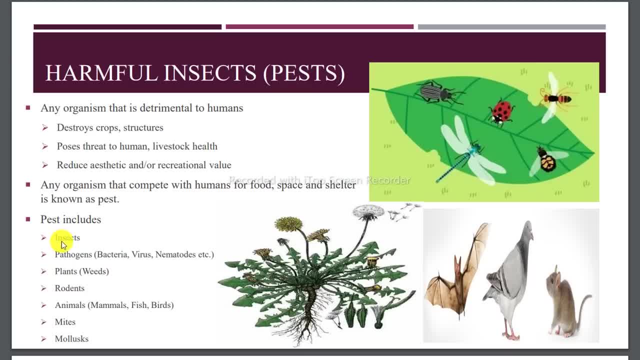 Pests include Insects. Insects include Pathogens, bacteria, virus, nematodes, Plants, weeds, Rodents, animals, Mammals, fish, birds, Mites, mollusks, Bats, Pigeons, Rats, Animals- Organisms That live in the environment. 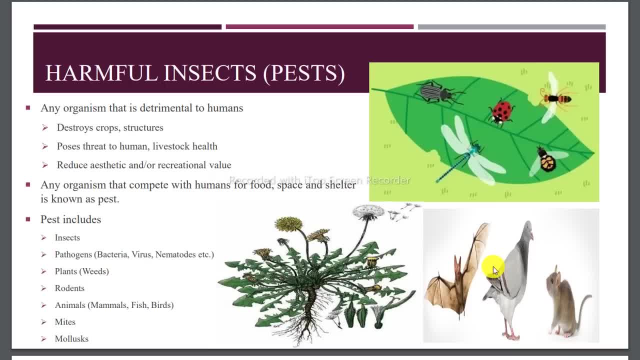 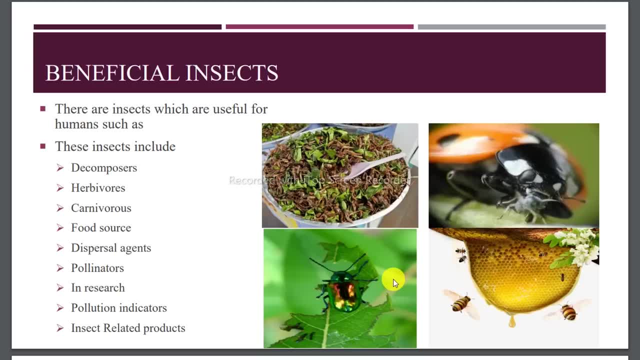 And these are the pests. Next Beneficial insects: There are insects Which are useful for humans, Such as Decomposers. Herbivores, Carnivores. Food source, Dispersal agents, Pollinators, Insects. Insects Which are useful for humans, Such as Decomposers. 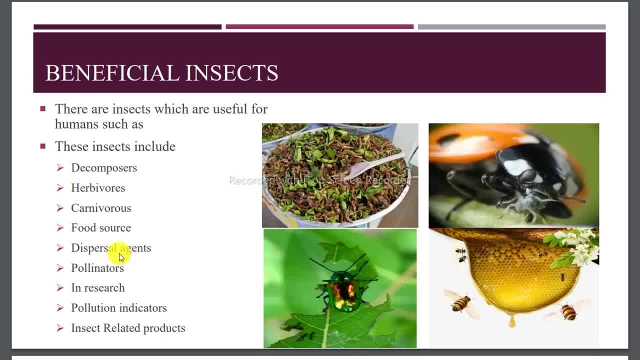 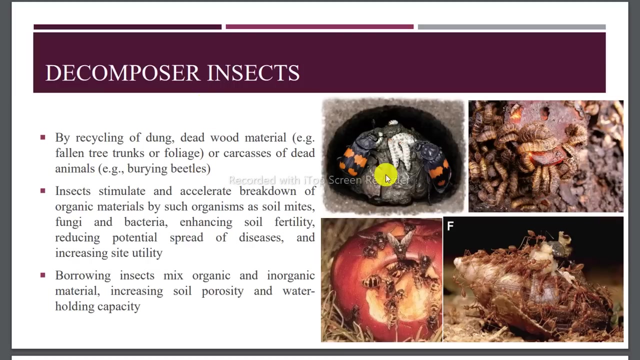 Herbivores, Carnivores, Food source, Dispersal agents, Pollinators, Insects. Subtitles: Polluci клins, Affection, Decomposer Insects. Insects eat decomposed things. like, If any of our fruits are spoiled, we throw it away and rot, then these people eat it. or, as I give you an example, that anything that is bad, like the part of the human body, if it is spoiled, then its property is lost, then these are the insects that eat decomposed things. 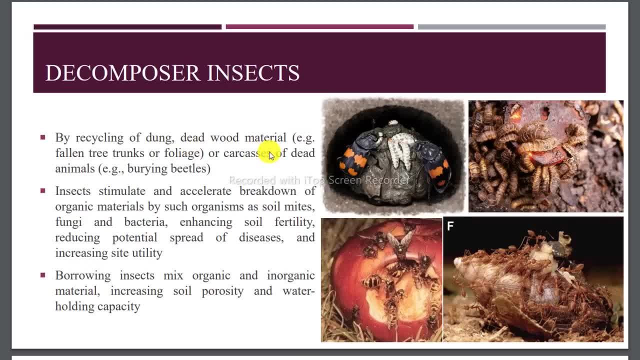 So by recycling of the dead wood material, for example trunks of foliage or carcass of dead animals burying beetles. okay, he is telling that the dead animals eat meat and eat many things that are dead or decomposed. 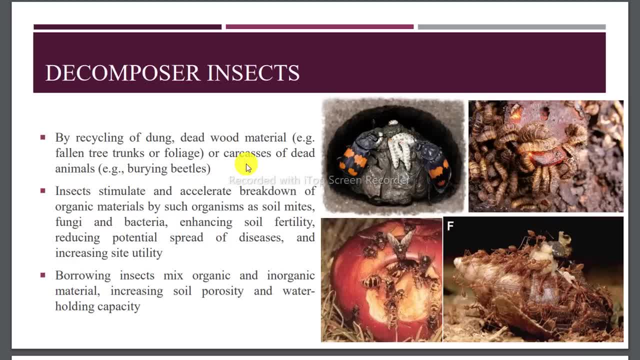 They eat those things And because of that, Insects stimulate and accelerate the breakdown of organic material by such organisms as soil mites. He is telling that insects stimulate and accelerate the breakdown of organic material that lives in the soil. The insects that live in the soil stimulate and accelerate the breakdown of organic material. 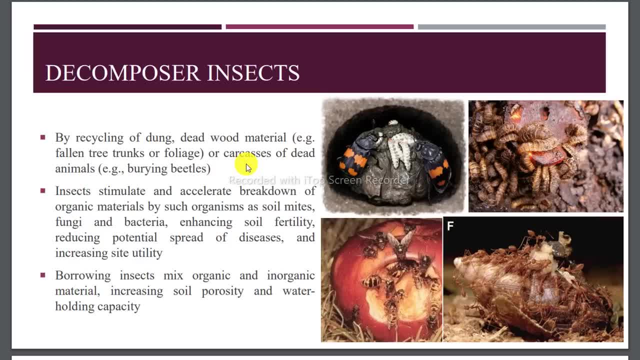 Okay. Insects stimulate and accelerate the breakdown of organic material and the soil mites. This is the structure of the soil mites And they are getting used to it. Now this is my second method to know about these insects, So I will show it to you again. 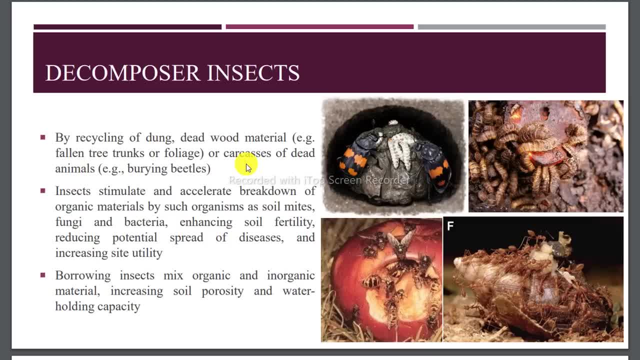 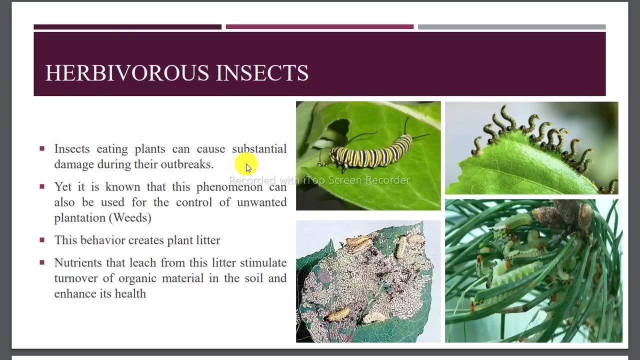 Okay. Insects mix organic and inorganic material, increasing soil porosity and water-holding capacity. Insects and insects increase soil porosity and water-holding capacity of soil. The third is herbivore insects. Insects can cause sustainable damage during their outbreaks. 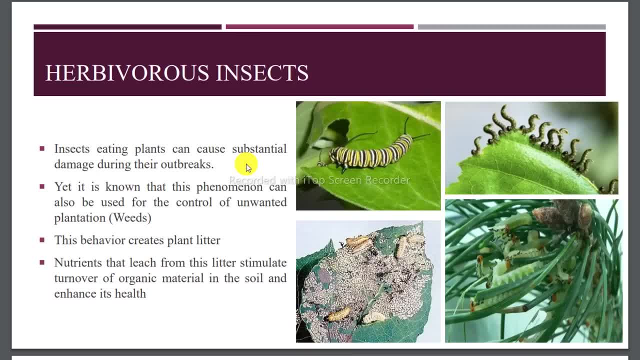 Second is that it is known that this phenomenon can also be used for the control of unwanted plantations. Insects and insects mix organic and inorganic material, increasing soil porosity and water-holding capacity. Insects and insects mix organic and inorganic material, increasing soil porosity and water-holding. 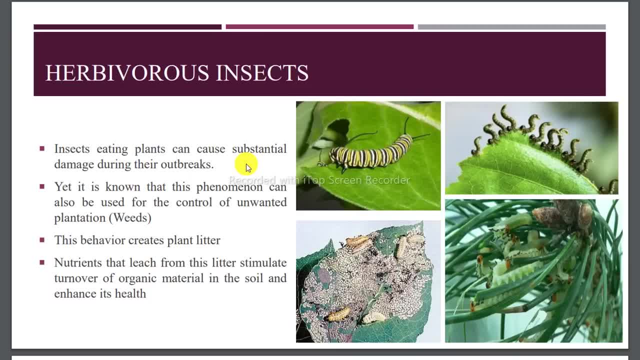 capacity. Insects and insects mix organic and inorganic material, increasing soil porosity and water-holding capacity. Plants in particular invasive. They increase the health of the soil because we get a lot of nutrients from them. So these are the insects that eat plants. 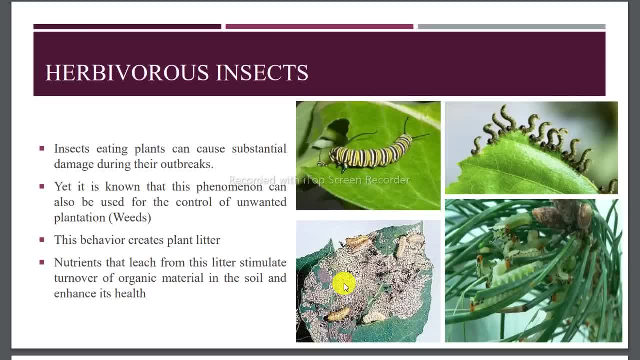 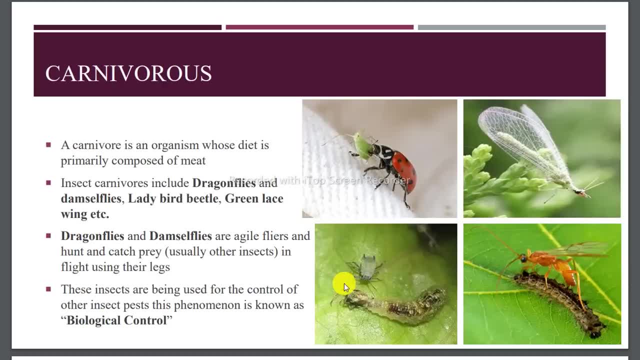 Let's go to the next slide: Carnivores. Carnivores is an organism whose diet is primarily composed of meat. These are carnivores whose diet is primarily composed of meat. Such carnivores include dragonflies, damselflies, damselflies, ladybird, beetle, green, lace, twink, etc. 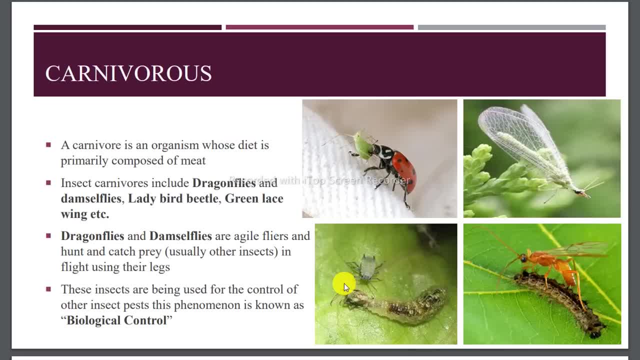 Second, dragonflies and damselflies. Damselflies are agile flies and catch prey, So these insects are often used to attack humans and other animals. Thirdly, these insects are used for the control of other insects' pests. This phenomenon is known as biological control. 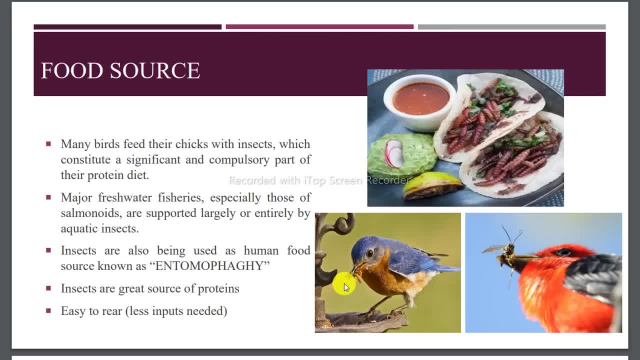 Fourthly, birds feed their chicks with insects, Which constitute a significant and compulsory part of their protein diet. What do birds do? They feed their chicks with insects. I hope I'm not making a mistake. I don't know what it is as a kid. 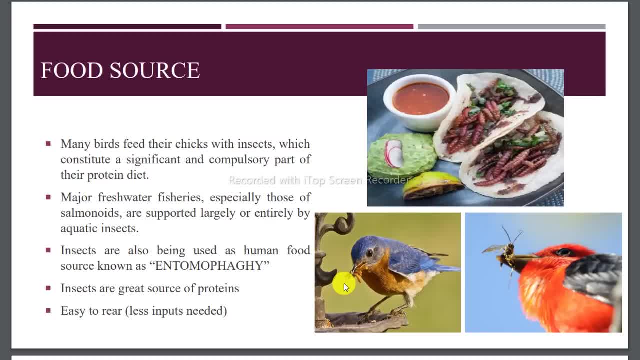 The second major freshwater fisheries, especially those of salmonides, are supported largely and entirely by aquatic insects. Insects are also being used as human food. Insects are a great source of protein. They are easy to rear and less impotent. They are easily found and do not require much expense. 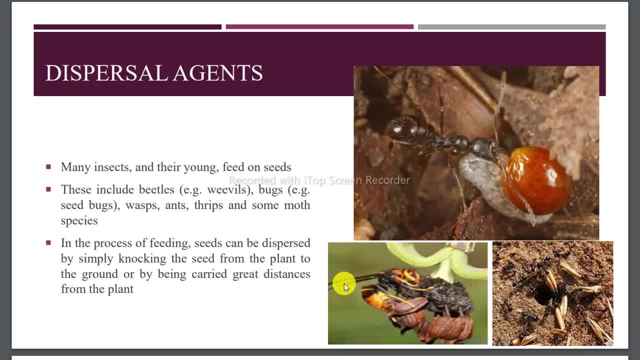 Dispersal agent. Many insects and their young freedom seeds, which are quite penseleic and have a lot of insecticides, are also known as disperse agents. Dispersal agents are also known as disperse agents. They are also known as disperse agents. 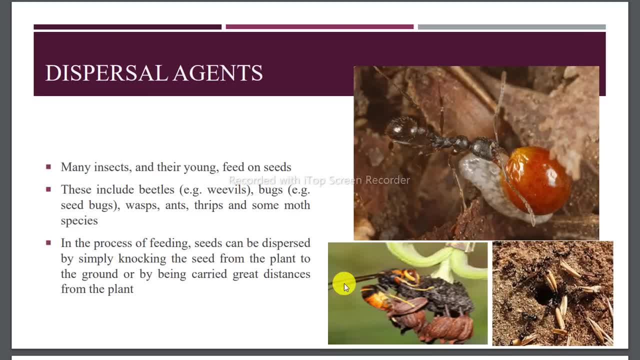 These insects and their children grow on the seeds. these include beetles, bugs, wasps, ants, thrips and some more species. All these are shown here in the images. these are ants, bugs, beetles. they eat all the seeds. 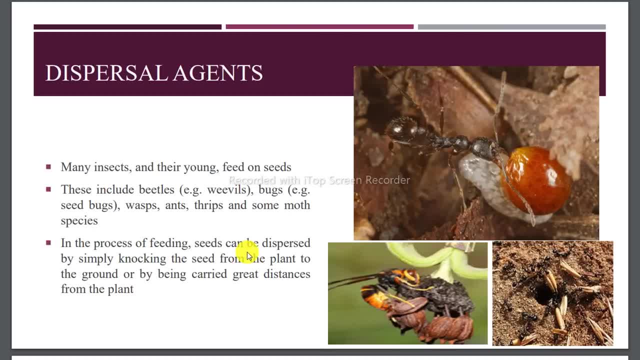 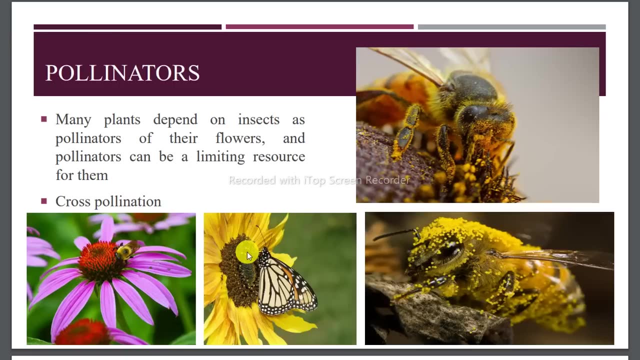 In the process of feeding. seeds can be dispersed by simply knocking the seed from the plant to the ground or by being carried to great distances from the plant. Many plants depend on insects as pollinators of their flowers, and pollinators can be a limiting resource for them. 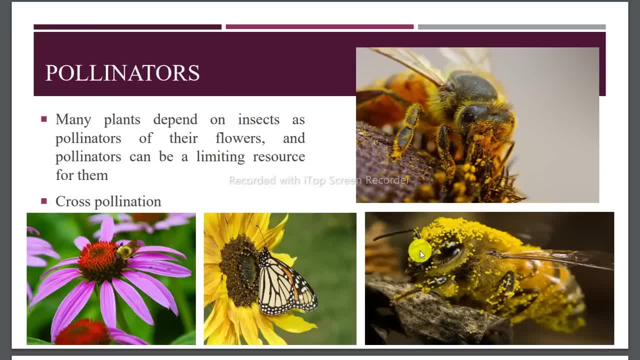 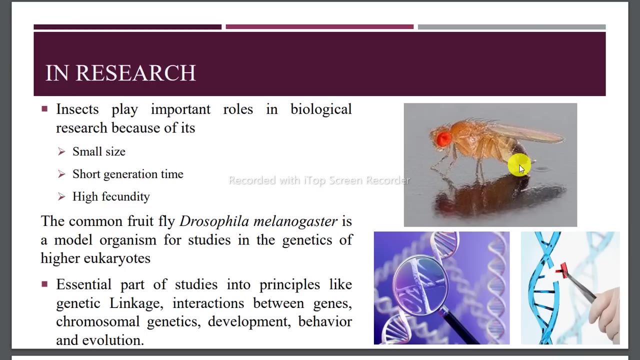 For example, we take the example of honey. honeybees produce honey for us. There are many such insects that come up in many new varieties of plants through pollination. Thank you. Insects play an important role in biological cells because of its short generation time, high frequency, small size.